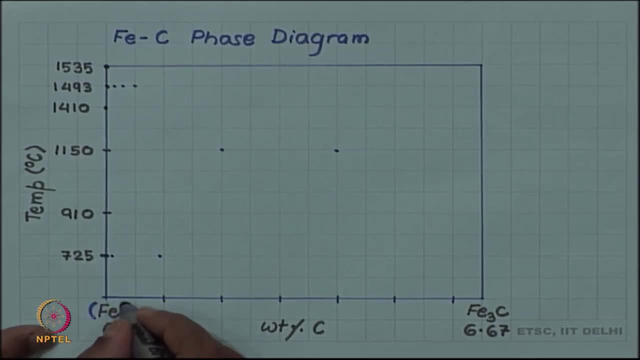 And since we are looking at iron carbon phase diagram, one of the ends is iron, which is 0 weight percent carbon. but this diagram is different from other diagrams which we have discussed, So the heat dissipation axis does not go all the way up to 100 percent carbon. we 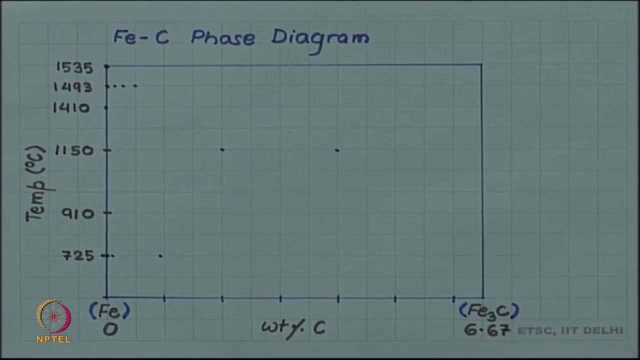 stop at all traditional iron carbon phase diagram. stop at F E 3 C, which is an intermetallic compound and its weight percentage is 6.67.. If you think of its atom percent you can see there is one carbon atom out of 4 atoms. So it has 25 atomic percent carbon in it. but 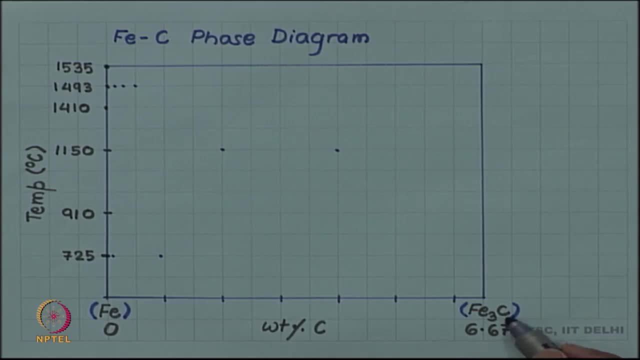 since carbon is lighter, 25.. atomic percent carbon contributes only 6.67 weight percent Beyond Fe 3 C. the diagram is not interesting to engineers because structure, the alloy will be too brittle and has no, not much engineering applications. So we look at this. so sometimes because of this, the iron carbon phase diagram also. 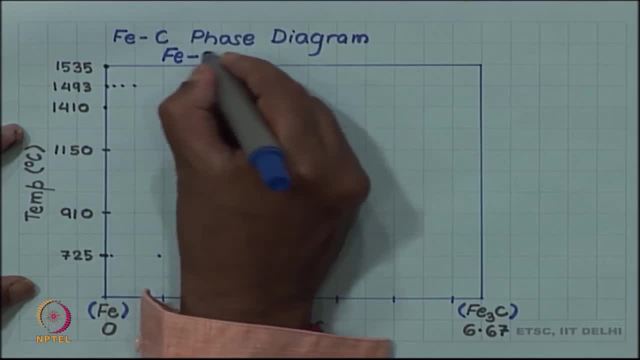 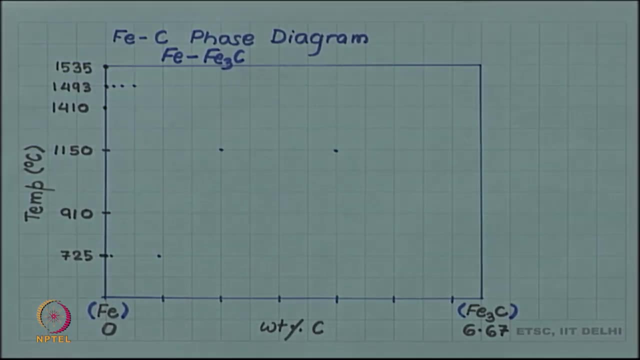 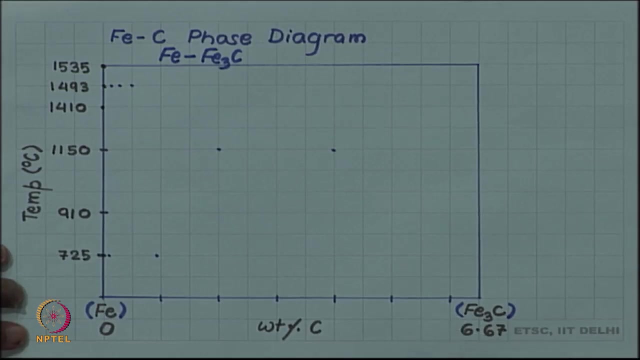 is called Fe 3 C diagram. iron carbide phase diagram is also sometimes used to indicate that we are ending at Fe 3 C Now. I told you that there are three invariant reactions and we have seen in the last video that every invariant reaction in a binary phase diagram 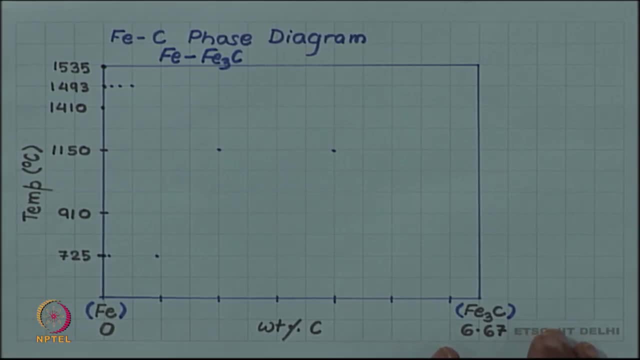 is always Represented by a horizontal line, so we will have three horizontal line. So let me begin with that. I am gradually trying to build up the phase diagram, because the phase diagram is complicated and seeing it all at once can be little unsettling to. 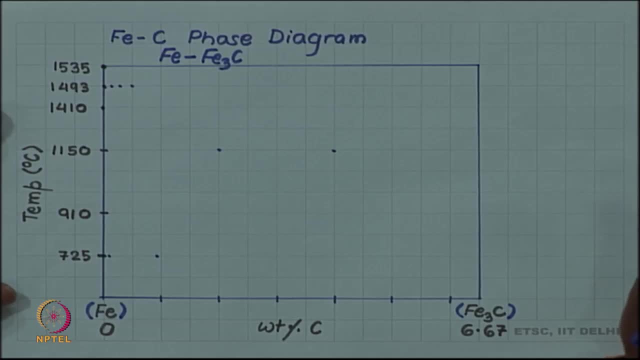 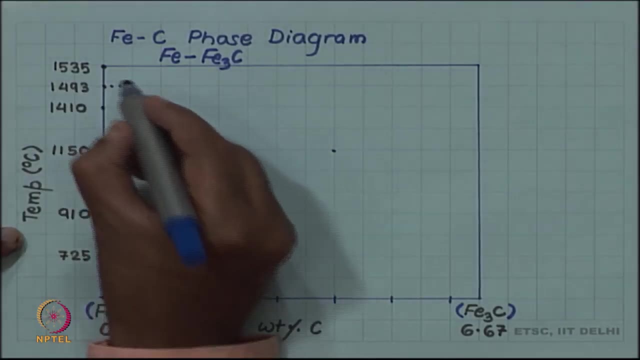 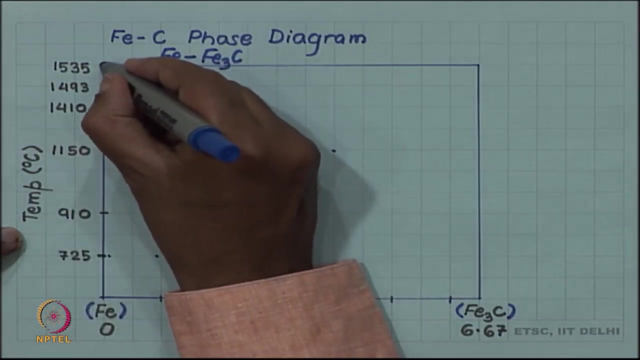 a beginning student. So we let us gradually begin with the each of these invariant reaction. the invariant reaction at highest temperature happens at 1493.. So I have three points there. 1535 is the melting point of iron. so that is an important point above. that is a liquid iron for pure iron. for pure iron, 1535 is the melting point, then 1410 is a solid state transformation and 910 is another solid state transformation. we will talk about that, So let us start with that. 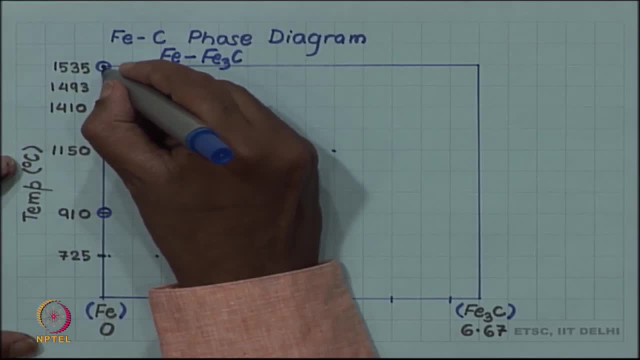 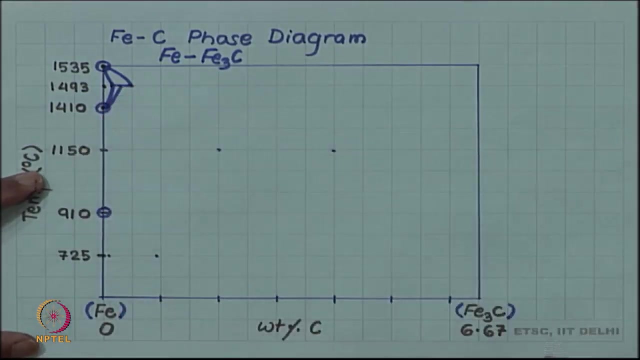 So I have three points there. 1535 is the melting point of iron, so that is an important point above that. So let me first complete this invariant reaction. so there is a phase boundary like this, then it connects with 1410.. 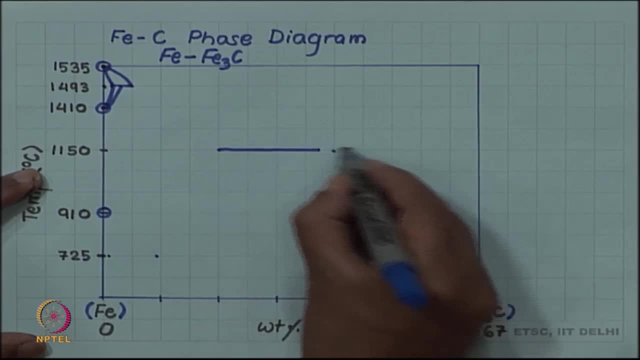 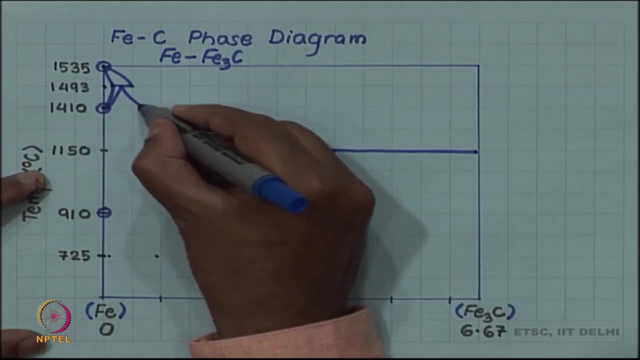 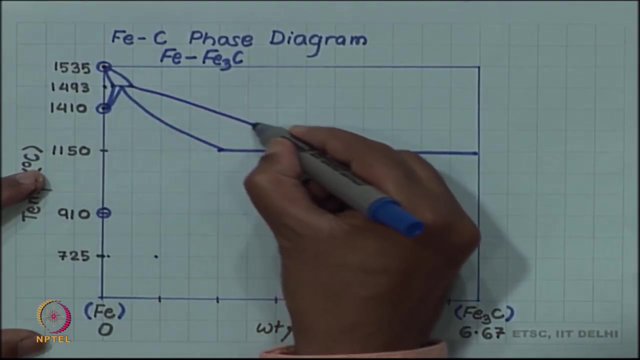 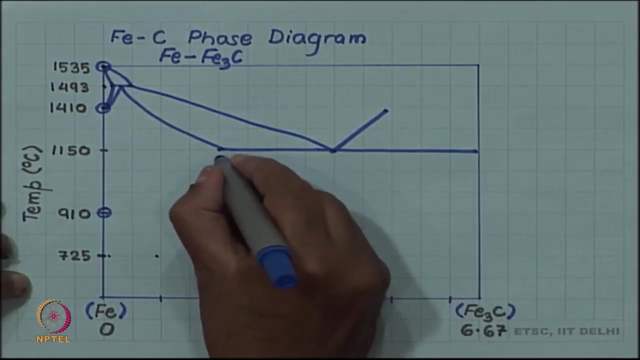 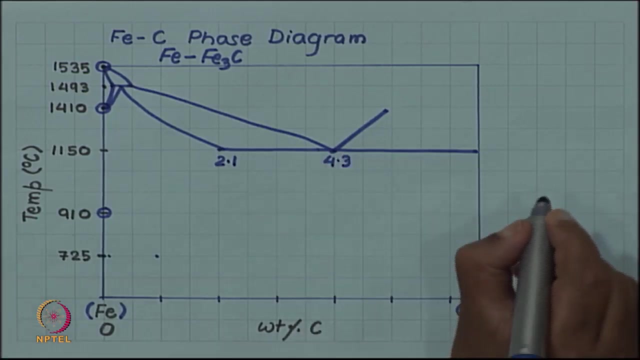 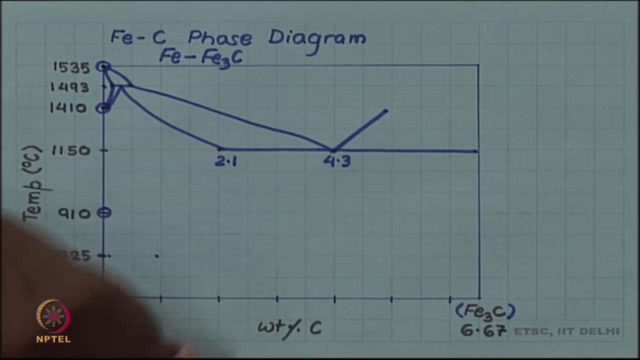 The another invariant reaction runs here. Okay, Okay, Okay. So there are phase boundaries connecting these two invariant reactions. This is 2.1 weight percent carbon, this is 4.3 weight percent carbon and here, of course, the compositions. 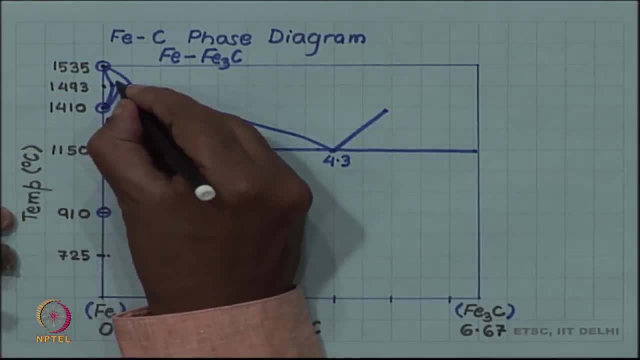 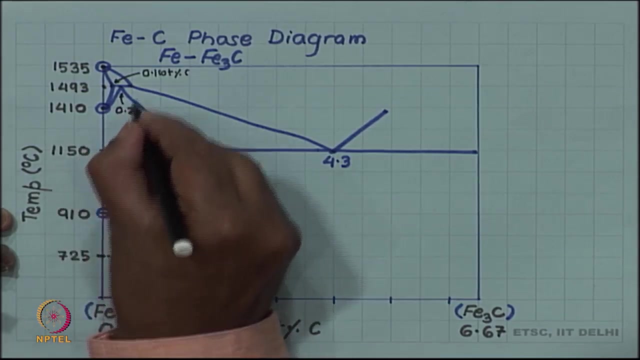 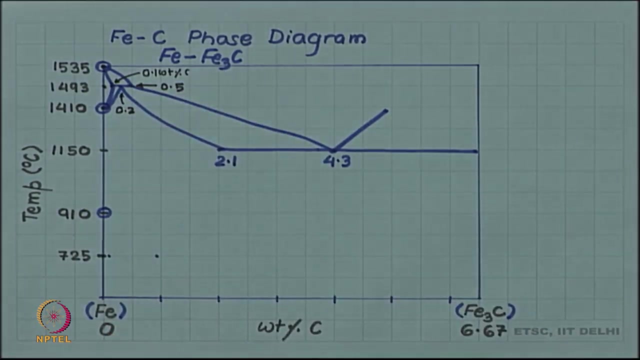 The compositions are little difficult to indicate, but let me try to indicate. that is 0.1. weight percent carbon, this is 0.2 and this is 0.5 and the horizontal temperature is 1493.. So that is one of the invariant reaction. 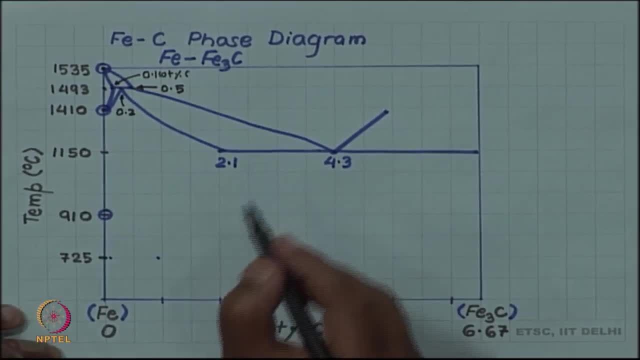 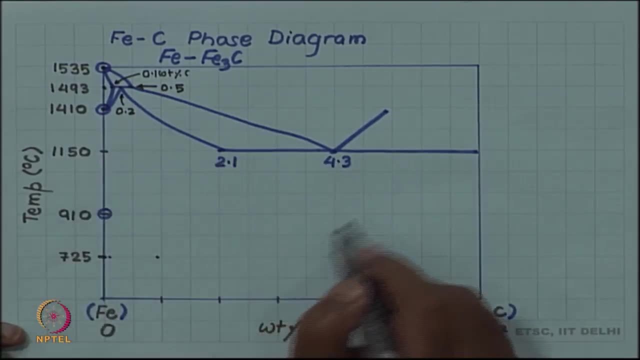 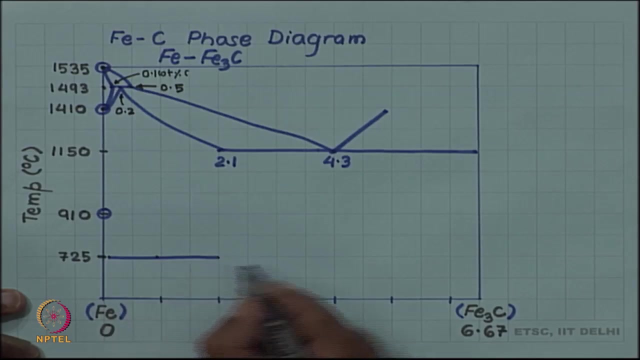 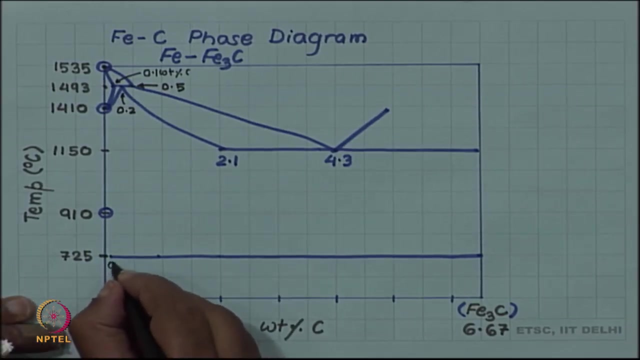 Then we have the next invariant reaction at 1150 degree Celsius, which is shown there, and finally we have an invariant reaction at 725, which has another horizontal line running here. its end compositions, the left hand composition, is very close to pure iron. 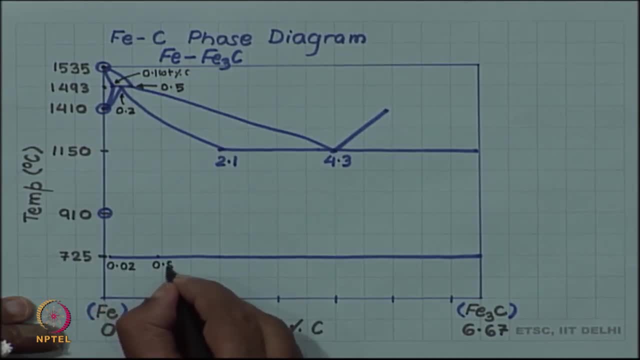 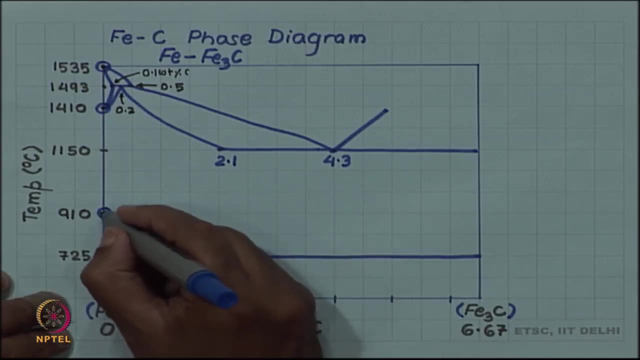 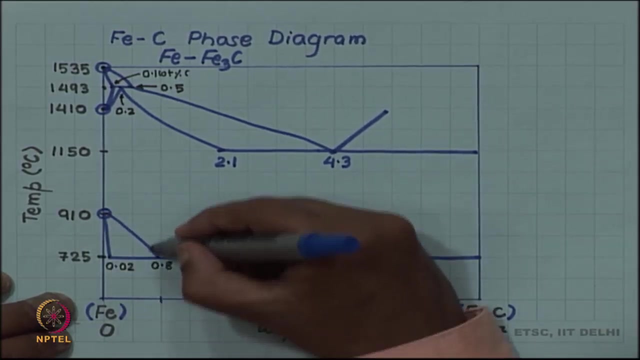 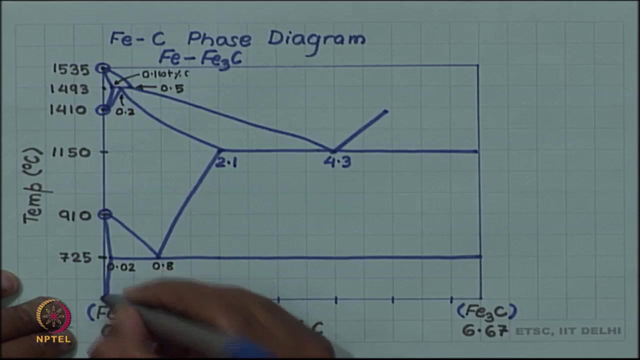 0.02.. Then this is 0.8, and it goes all the way up to 6.67.. So let me now connect these. you have boundaries here like this and boundary running from there and a final boundary coming here. 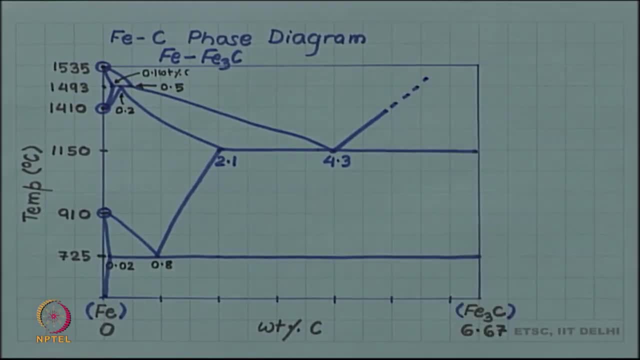 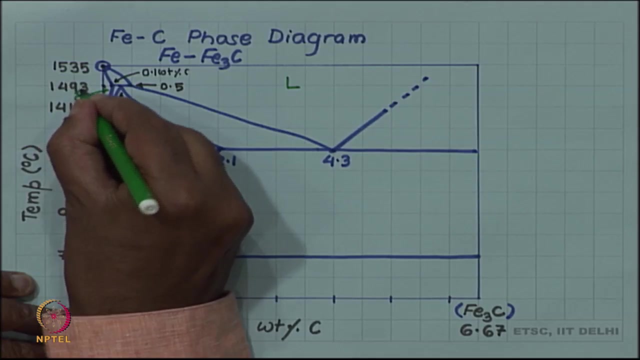 So this now completes the phase diagram. Let us write down the phases. This large region at the high temperature region is the liquid region. This small triangle here is what is called delta. each phase has a symbol as well as a name, So it has. it is delta. we will give you the name. 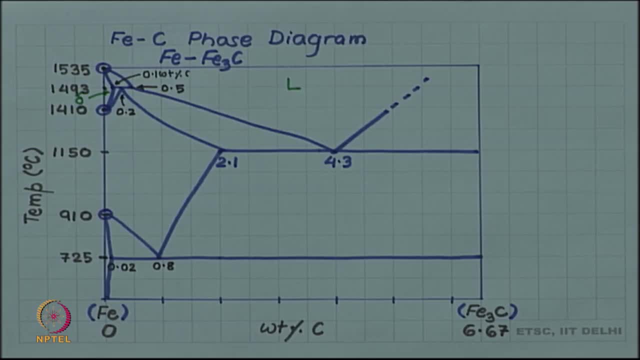 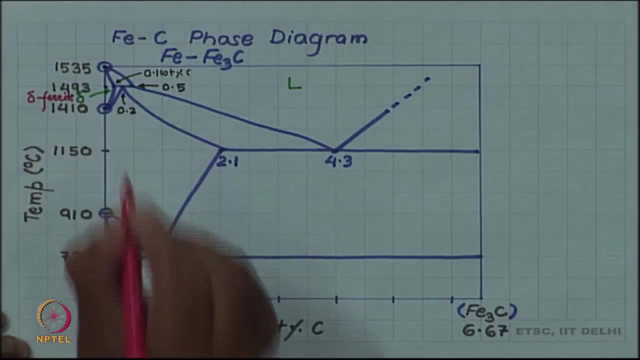 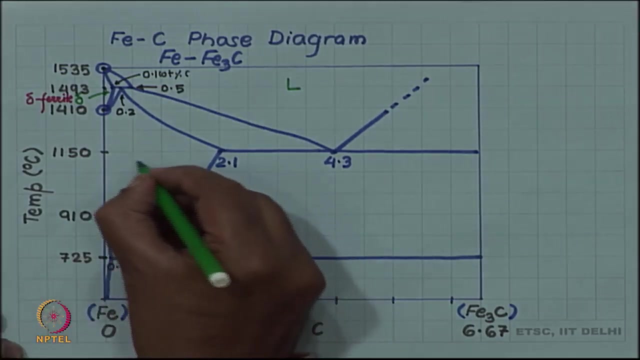 The name is delta. The name is delta ferrite. Name is delta, ferrite symbol is delta. Then this is a single phase region. this large single phase region, very important region, is gamma. This is called austenite. Okay, 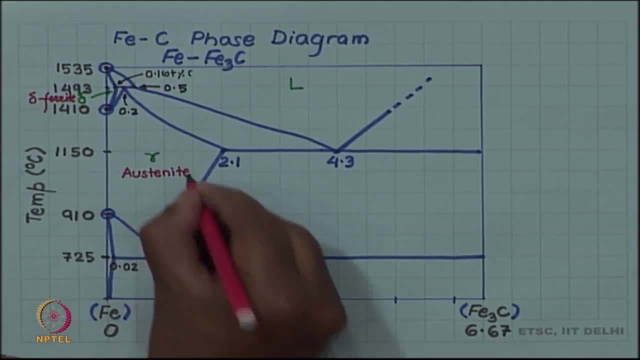 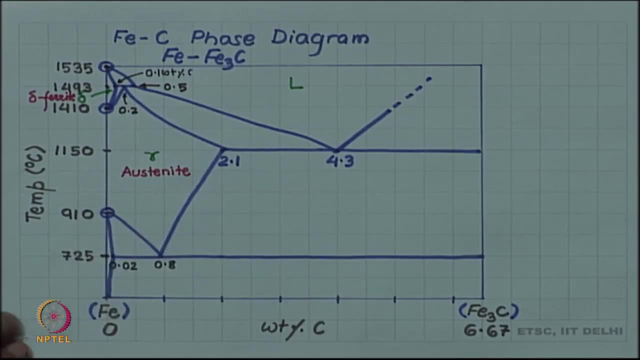 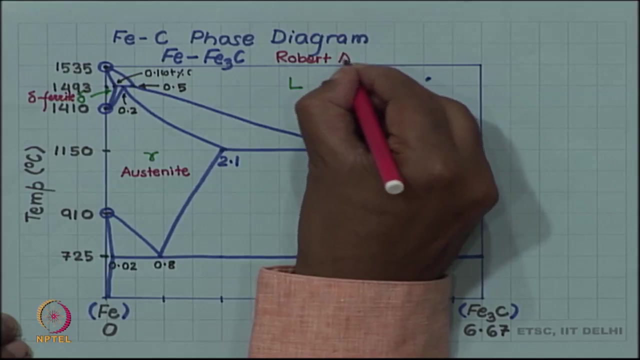 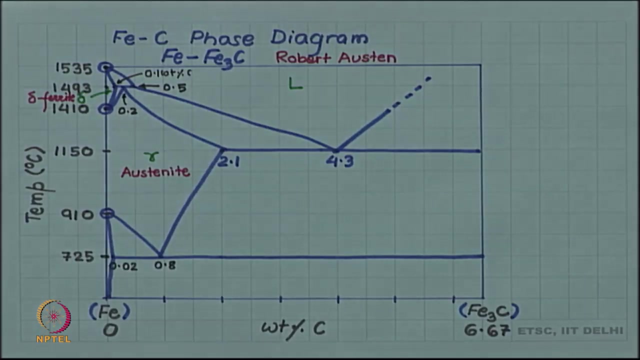 Okay, Okay, Okay, Okay, Okay Okay. This is named after the famous metallurgist who first made this phase diagram. that was Robert Austin. He was the first person to study iron carbon phase diagram, So in his honor, this large single phase region is called austenite. 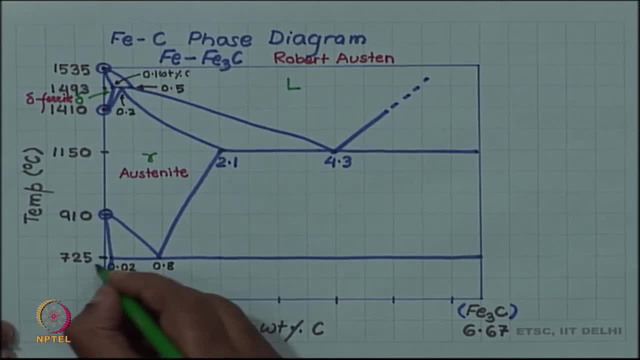 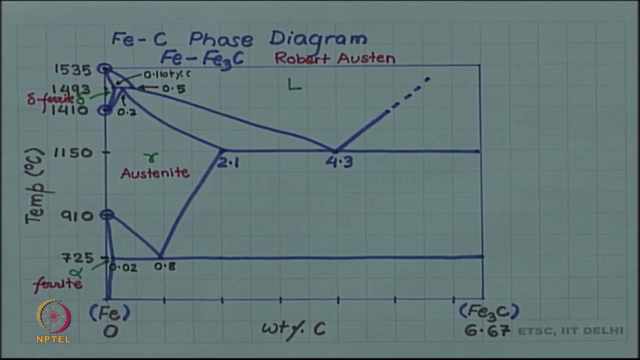 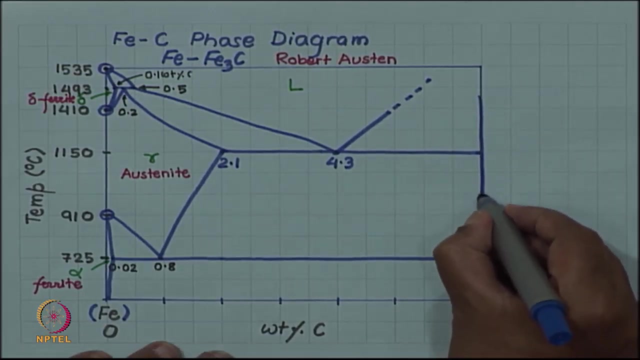 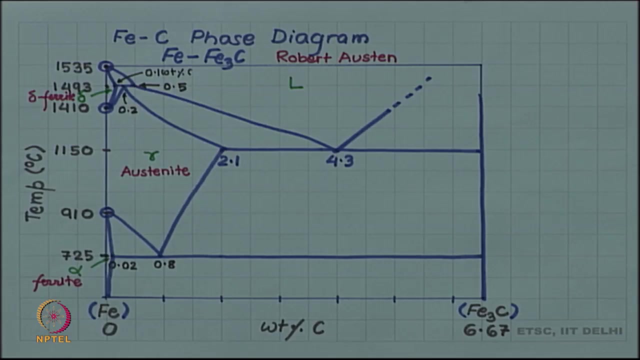 Okay, Okay, Okay, Okay. Then you have a small triangular region here. this is called alpha and its name is simply ferrite. Alright, And the vertical line here- this vertical line here itself is a phase- is a single phase region only, since it is a compound, it exists at a fixed composition, So it does not have 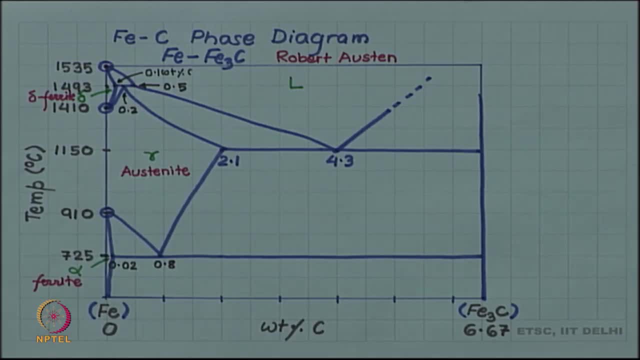 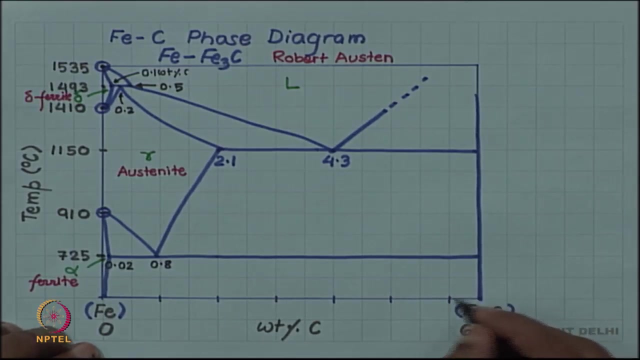 any width in the composition space, and this is So. this is also a single phase, this is a single phase region and this F e 3 C. the symbol is F e 3 C. the name given to it is cementite, cementite. So now you know all the single phase regions. 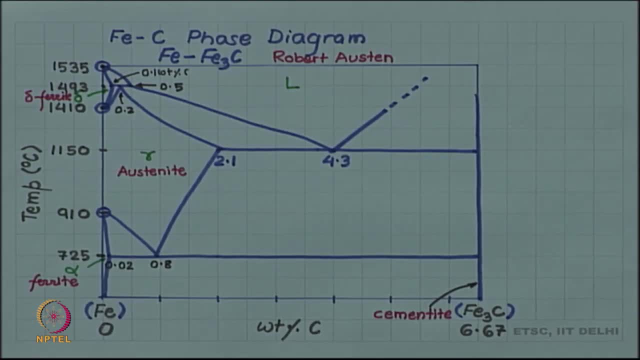 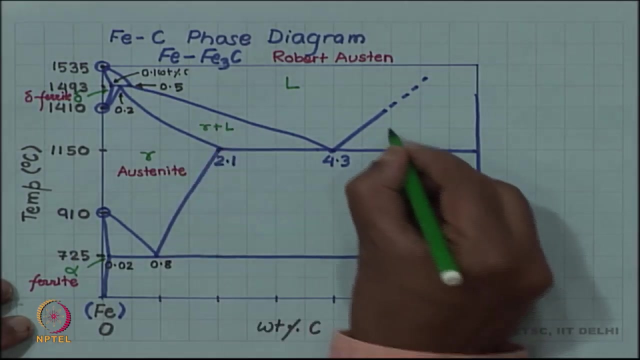 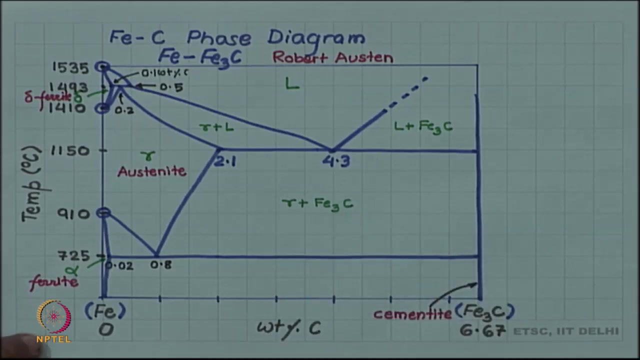 the two phase regions which I have known not labeled can be easily labeled. recall the one to one rule. So if you remember the one to one rule you can easily label all the two phase regions. So this region will, for example, will be gamma plus liquid, liquid plus Fe 3 C, gamma plus Fe 3 C, alpha plus. 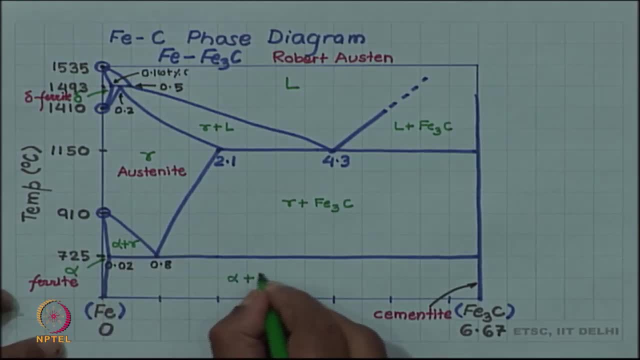 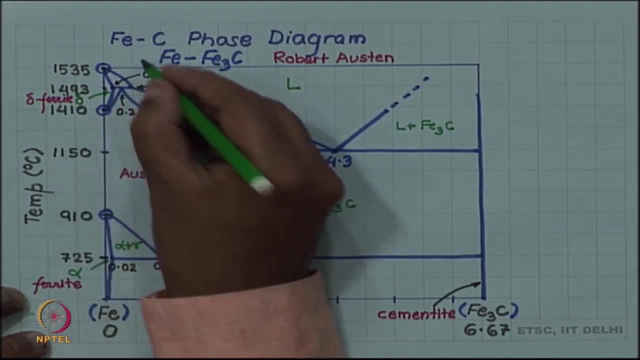 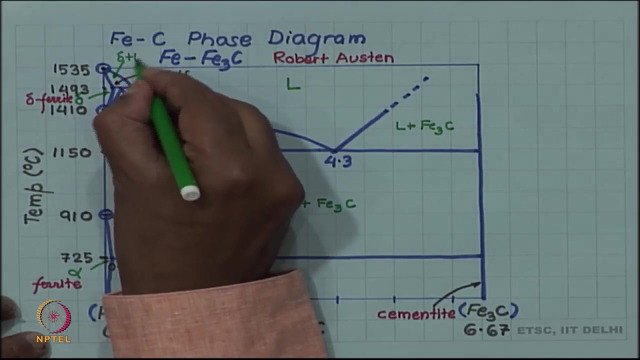 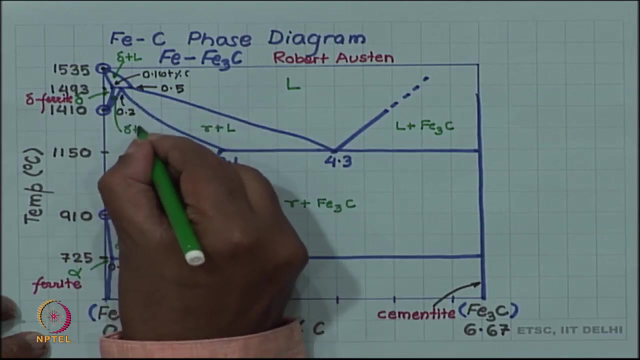 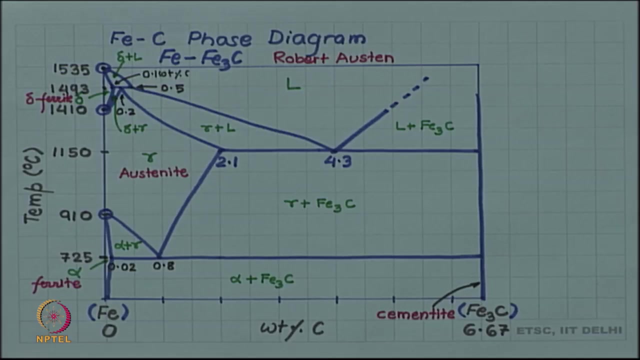 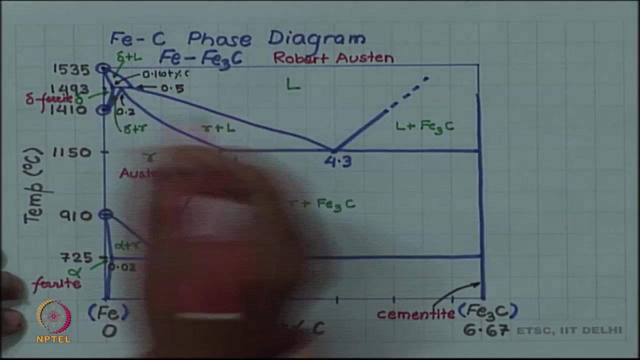 gamma and alpha plus Fe 3 C. The two phase regions here also can be labeled. space is not there, So this is between delta and liquid, this is delta plus liquid and this one there is delta plus gamma. Each invariant reaction is given a special name, So the invariant reaction happening at the two phase. 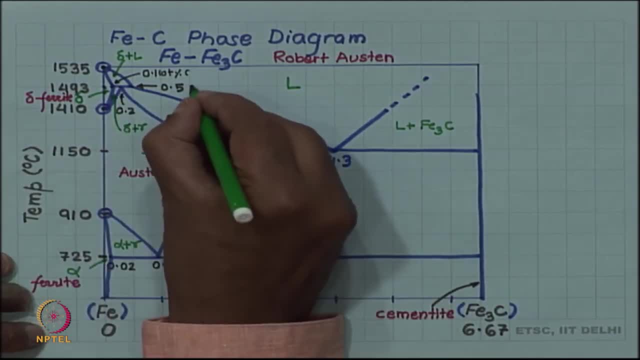 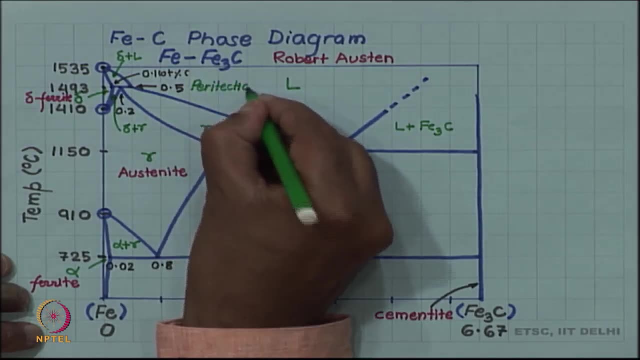 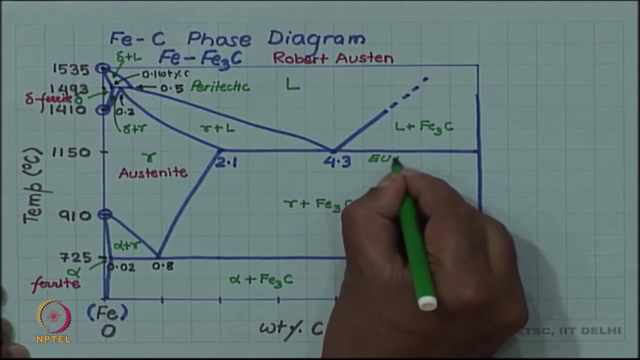 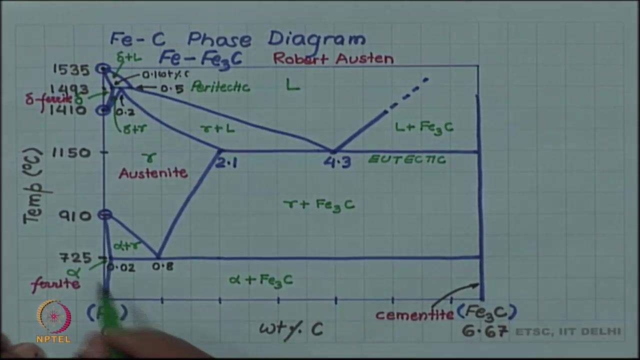 regions this temperature at 1493, this is called a peritectic reaction: peritectic, The one happening at 1150, you might recognize because you have met it. this is the eutectic and the one happening at 725 is the eutectoid. 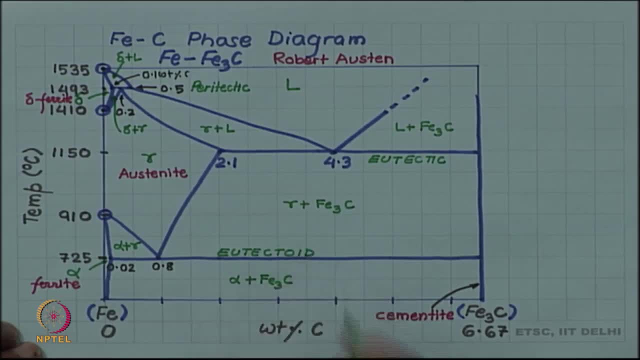 So this completes the diagram. we know all the compositions and temperatures, we know different phase regions, we know what phases are present in that and we know the names of the three important invariant reactions happening in this. Let us write down in full these invariant reactions. 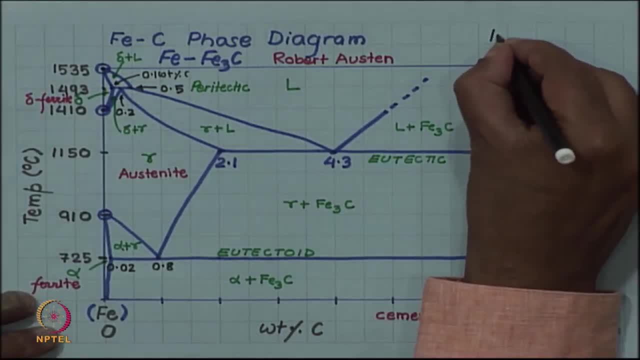 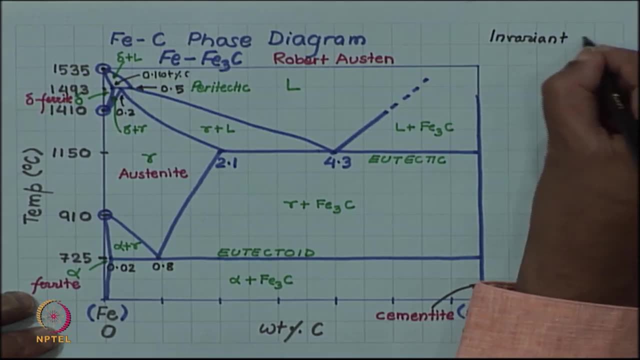 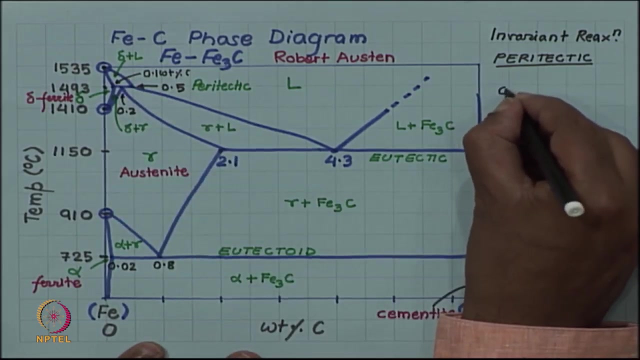 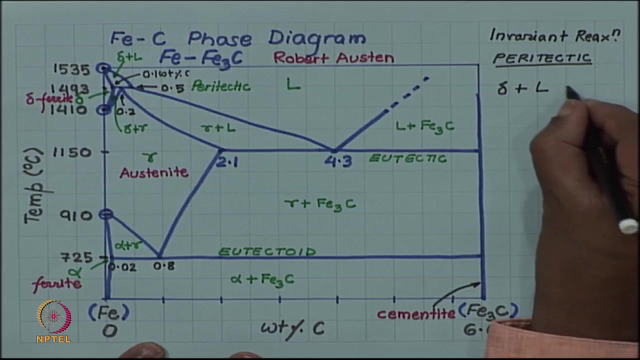 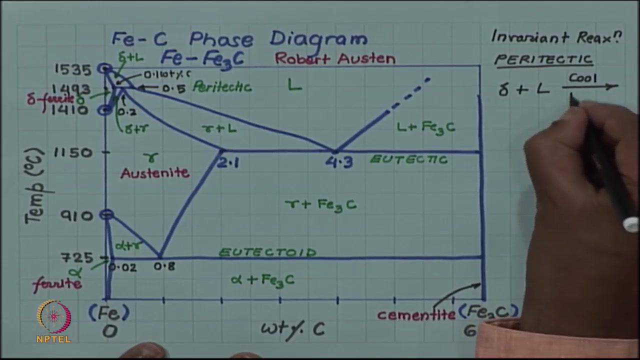 Invariant reactions. the first one, at the highest temperature, is the peritectic horizontal. you have delta plus liquid region. So you have delta plus liquid which transforms into on cooling. at a temperature of 1493, it will transform into a single-phase gamma. 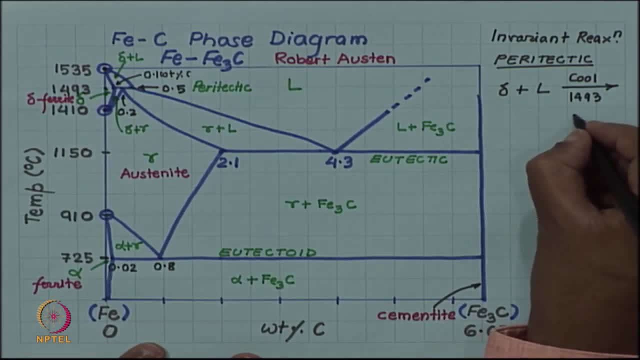 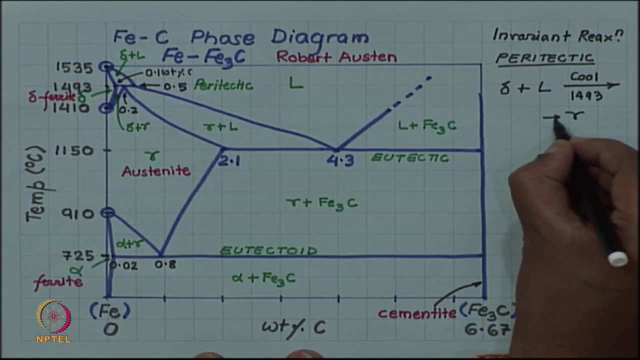 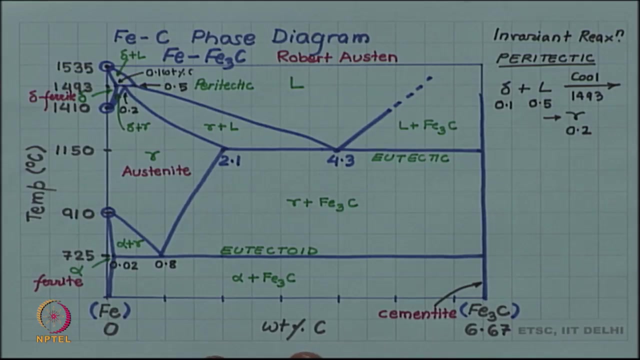 into a single phase. gamma Delta plus liquid on cooling is changing to gamma. The composition of delta is 0.1, of liquid is 0.5 and gamma produced is 0.2.. So that is the peritectic reaction. The eutectic reaction is happening at 1150.. 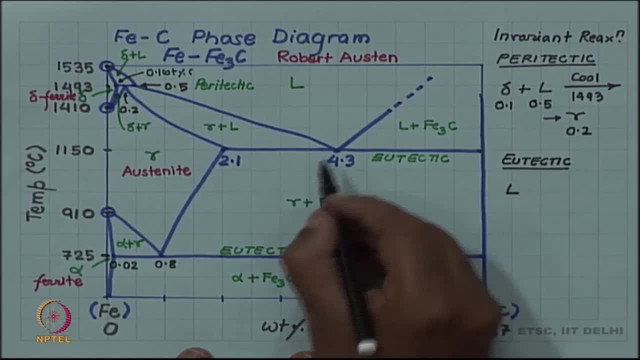 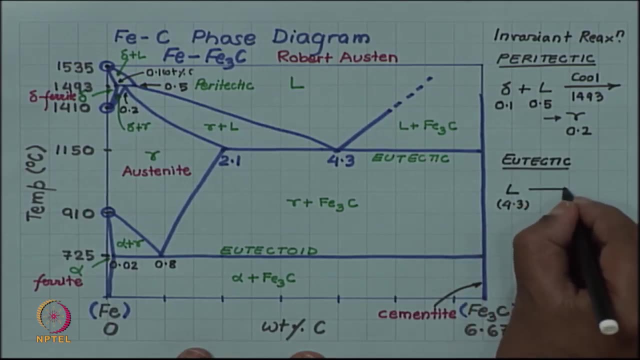 We can write this as liquid liquid. the higher temperature phase is the liquid of 4.3 percent. on cooling through 1150 degree Celsius will transform into two phase mixture of gamma and Fe 3 C. Gamma is gamma. composition is 2.1 Fe 3 C. we have already given 6.67.. 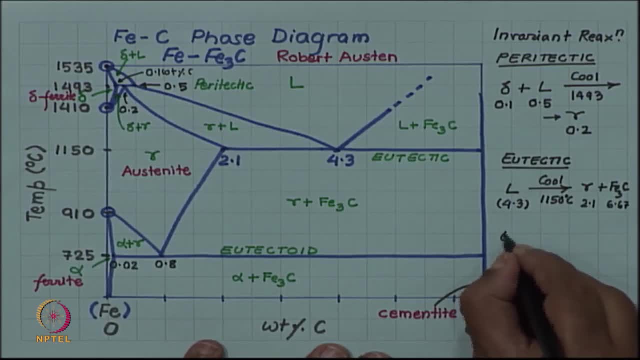 And finally the last one. here is the eutectoid. in this a single phase gamma of composition 0.8 decomposes on cooling at a temperature 725 into alpha plus Fe 3 C. So the alpha composition is 0.02. alpha is very pure ion and Fe 3 C is again 6.67.. 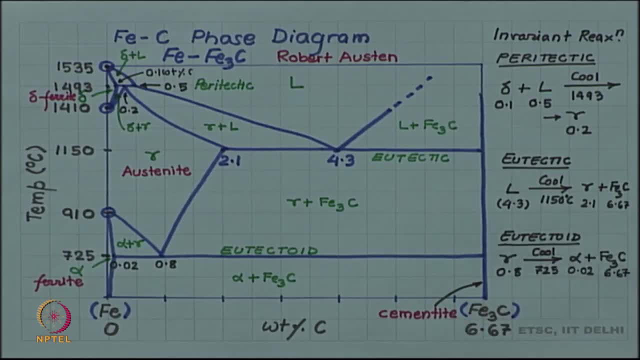 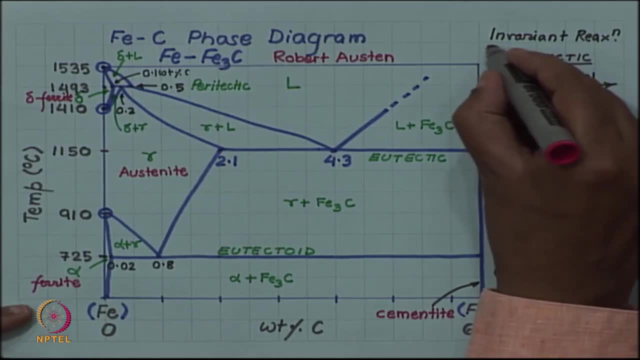 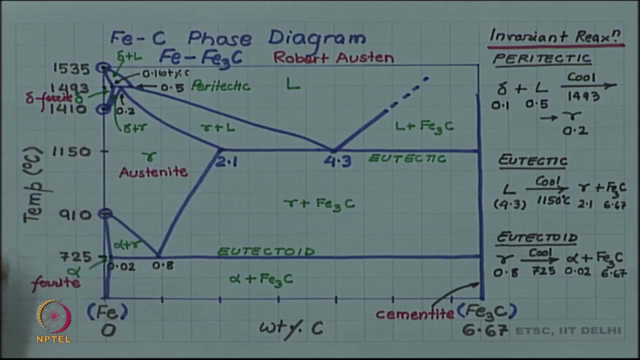 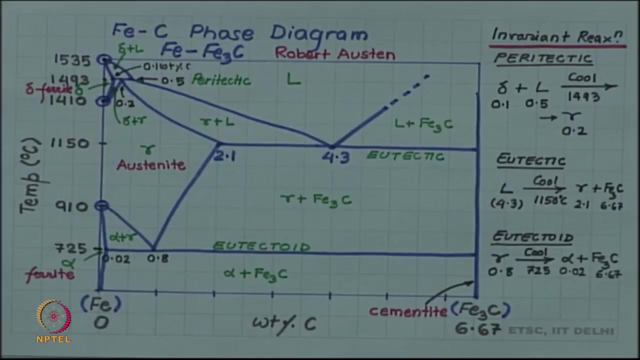 So now you know the details of all the three reactions, the invariant reactions, which are happening in this phase diagram. Let us look at little bit more about these phases, That what do we mean by phase diagram? So the phases in ion carbon system, and one more thing I want to say, two more things. 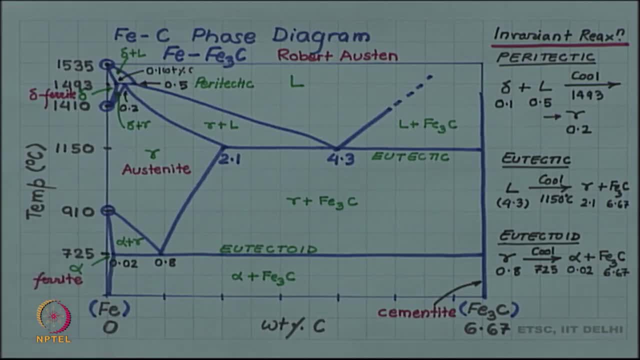 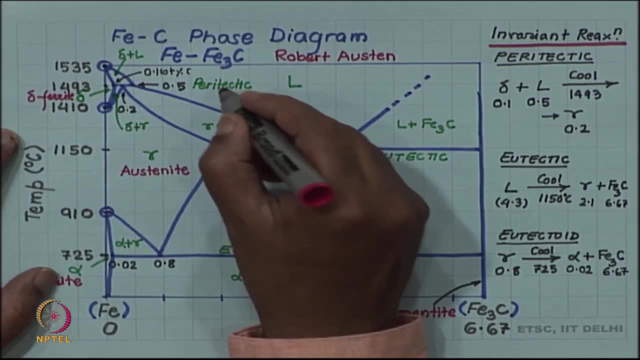 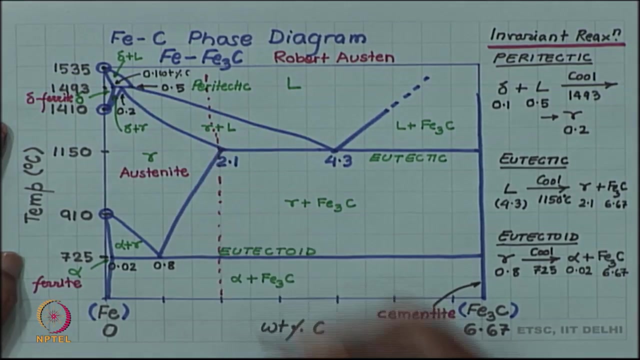 actually that in this diagram, if you look at compositions, less than generally a rough demarkation line, because we have two kinds of alloys of iron and carbon. one is called the cast iron, another is called steel Cast iron, so that means the ion is cast and another is called the Fe 3 C on cooling. 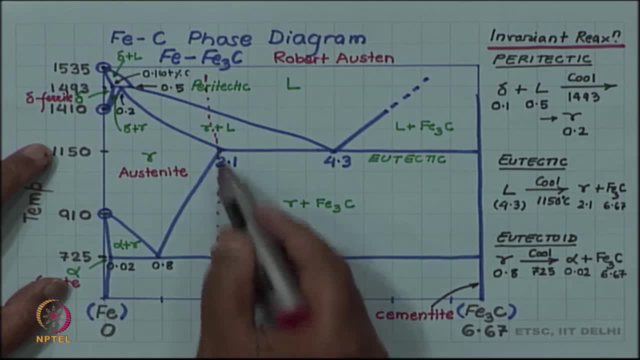 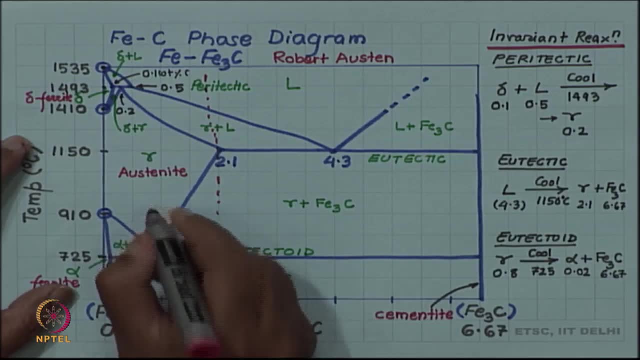 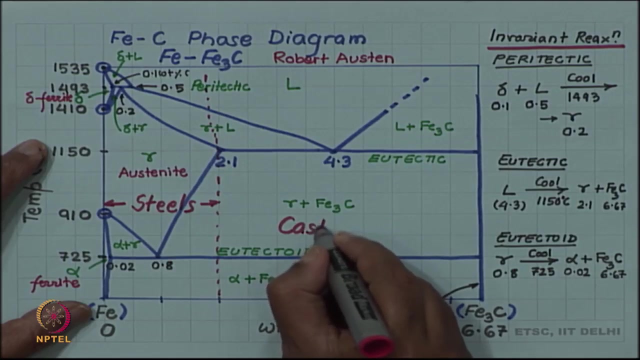 steel and a rough demarcation line is drawn at this point about 2 weight percent. So alloys less than 2 weight percent carbon, these alloys are called the steels, And alloys with higher carbon, these are called cast iron. You can see that: 4.3 percent carbon. 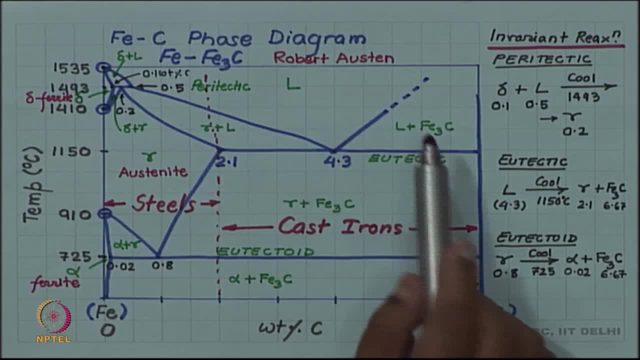 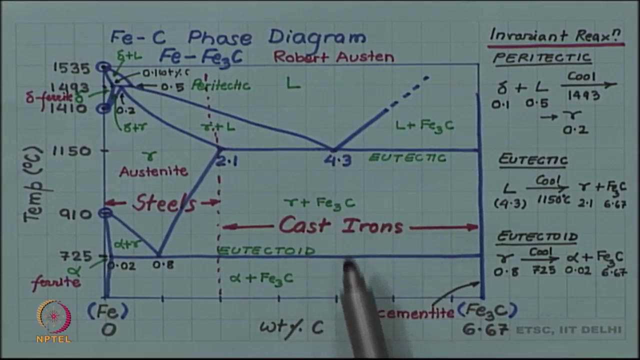 is a lowest melting point in the whole alloy system. So this: if you have 4.3 percent carbon, that iron carbon alloy will melt at a very low temperature of 1150 degree Celsius, And low melting is beneficial for casting, So the casting alloys are having higher carbon. 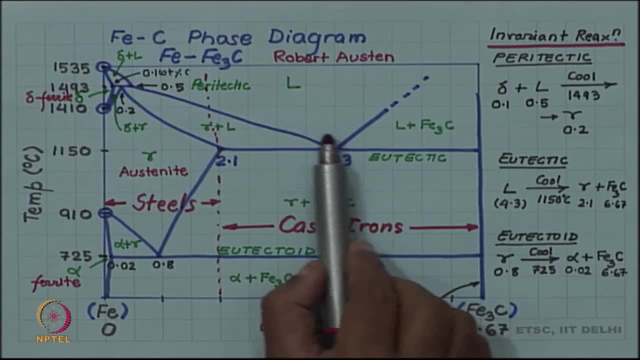 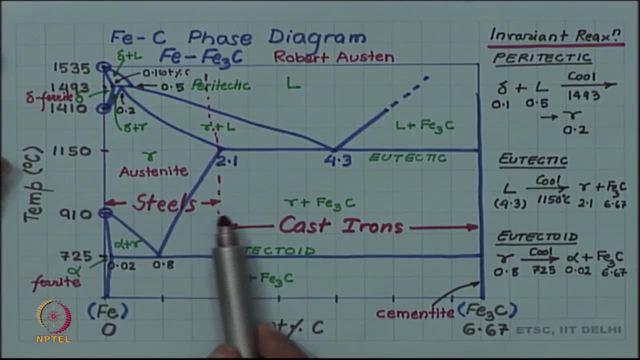 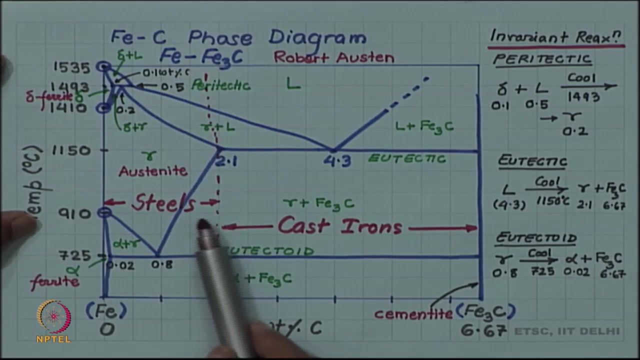 and so that they melt at a lower temperature Where steels during manufacturing it will melt one way in the steel melting furnaces, but after that in fabrication processes usually we do not melt it, we do not cast it to give different shape. So these alloys generally 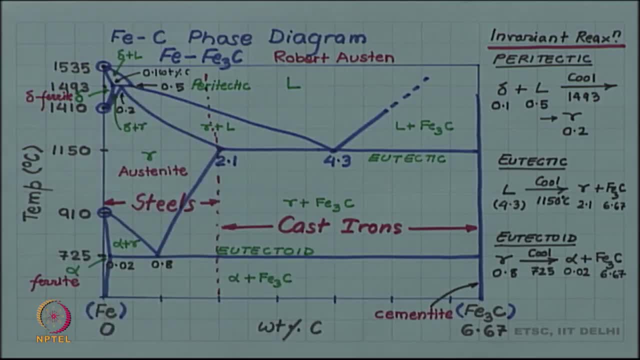 have higher melting point and it is not favorable for casting. And another important point which I wanted to talk is that this eutectoid reaction happens to be the most important reaction out of the three, So this has an important place. we will see why, because this is the control of the eutectoid reaction. is what 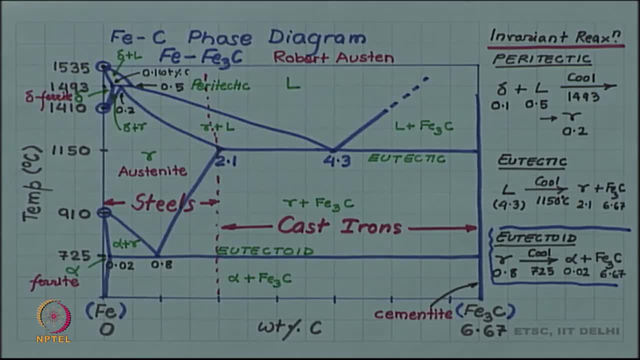 gives you the control on the microstructure of a steel through various heat treatments. So we will discuss that as we go along in this course. So because of that, it is not the full diagram which is of great interest to us, but the diagram close to this eutectoid. 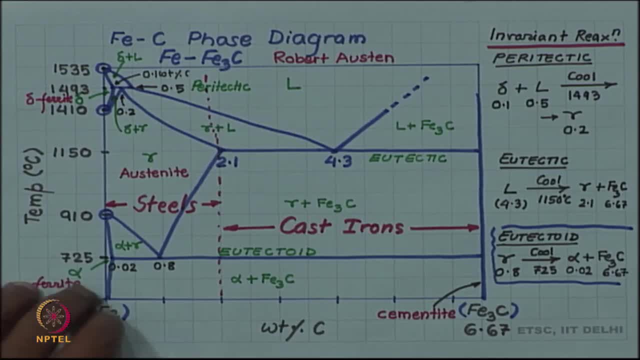 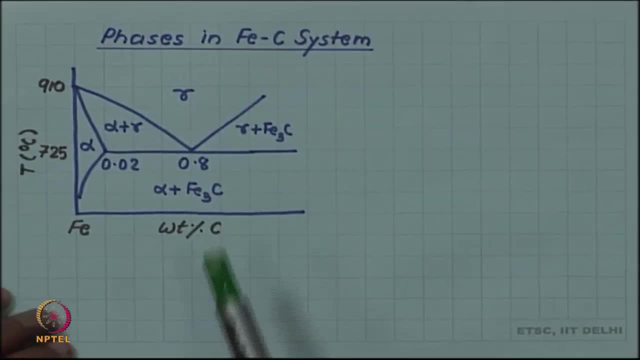 reaction is what becomes important, And that is why it is this part of the diagram which we will use fully focus, which is what I am showing you Here: only the lower part near the eutectoid, eutectoid composition. So let us look at. 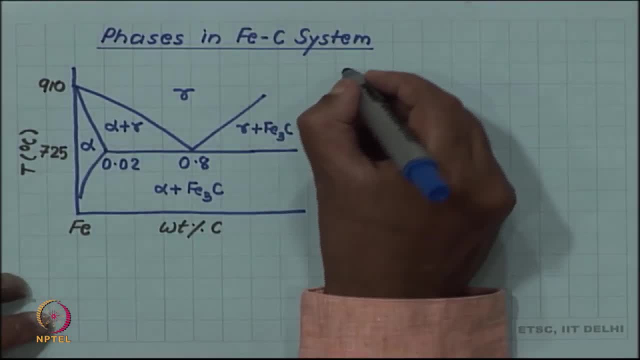 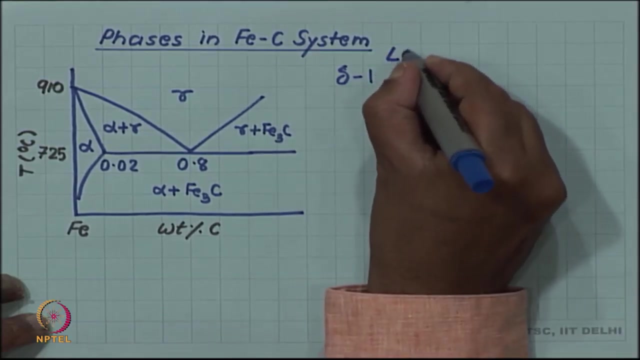 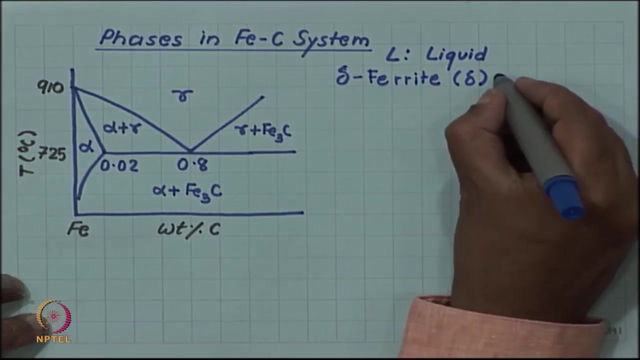 all these symbols and names again, of various phases. So you have, at the highest temperature not shown here, you have. you have delta ferrite, of course before also you have liquid. So you have liquid, then you have delta ferrite symbol is delta. 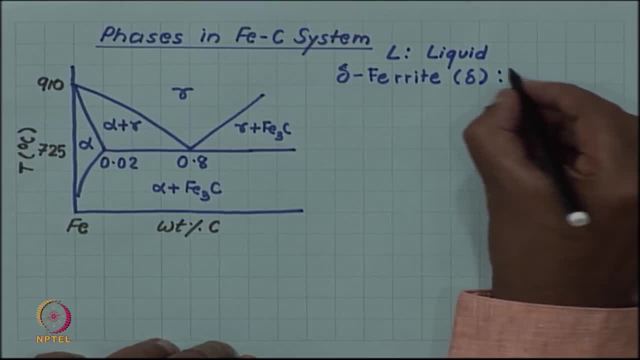 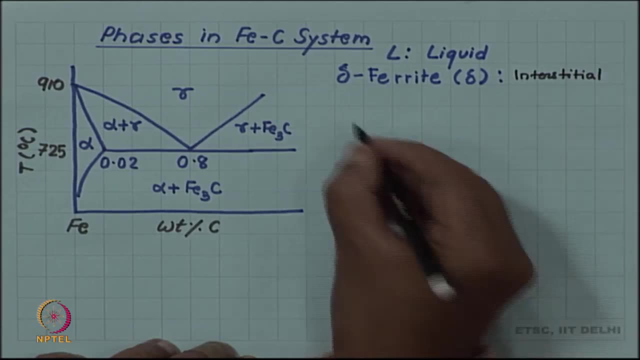 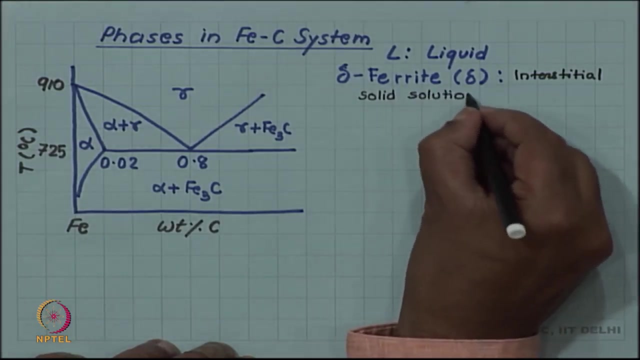 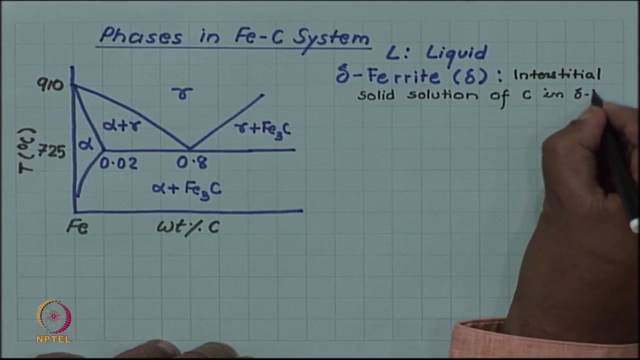 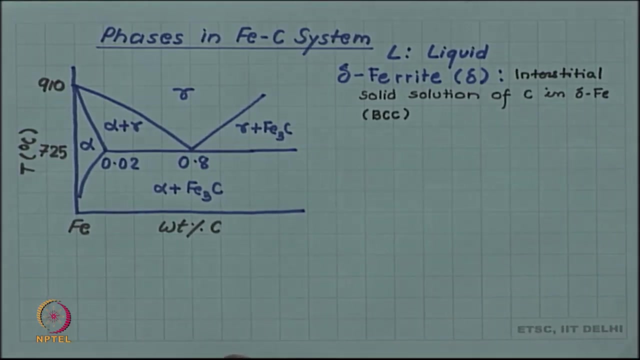 This is nothing but interstitial. interstitial. 2000, 2000, 2000, 2000. solid solution of carbon in delta ion. and delta ion is nothing but BCC form of ion at high temperature. You remember the look at the phase diagram, So delta was in this. 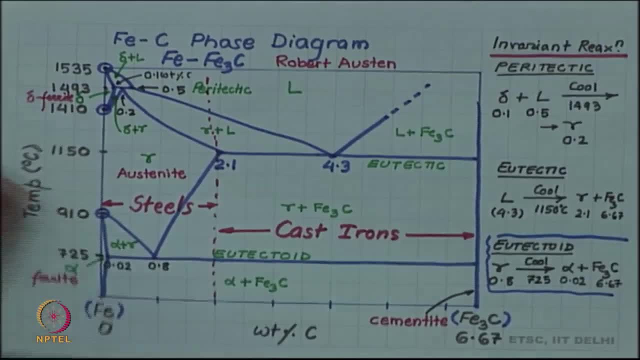 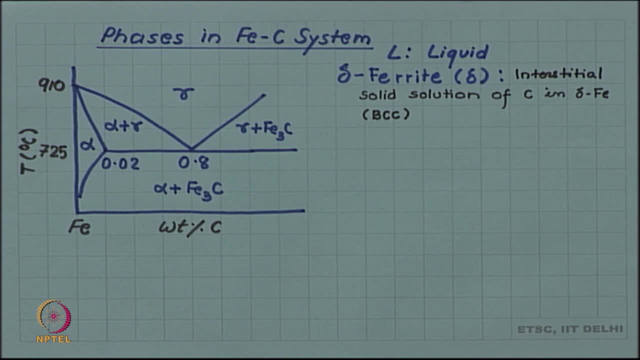 region, So it was a high temperature form and it was BCC, So that is delta ferrite, and it can have some carbon, So that carbon goes into the interstitial solid solution. Then you have gamma, which is also known as austenite. This is also interstitial solid. 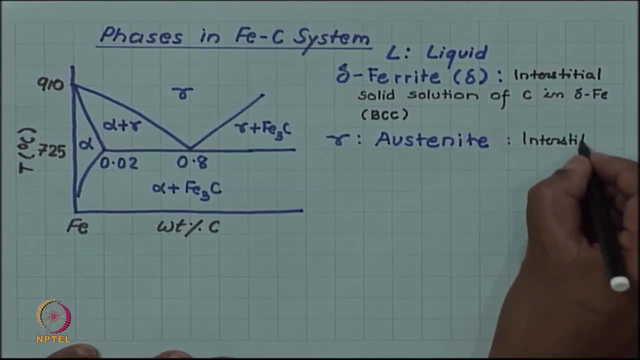 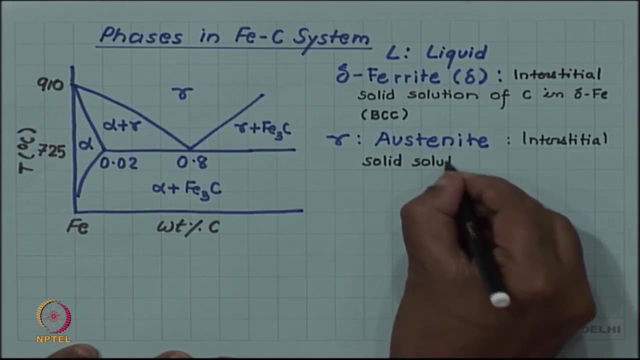 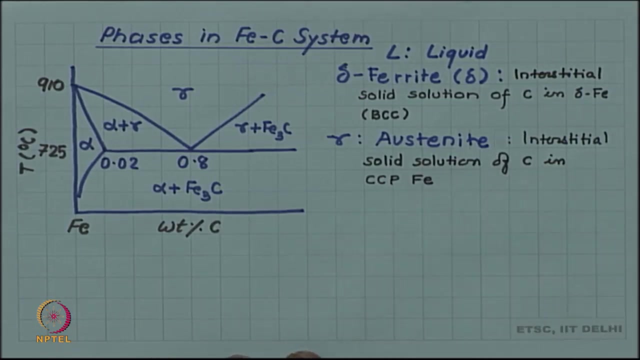 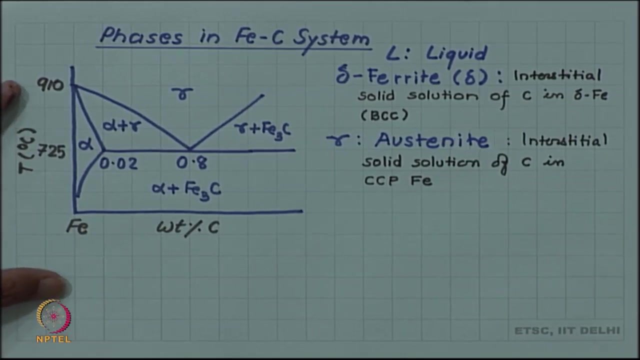 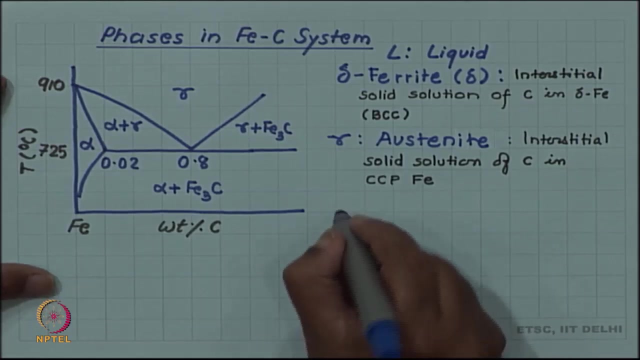 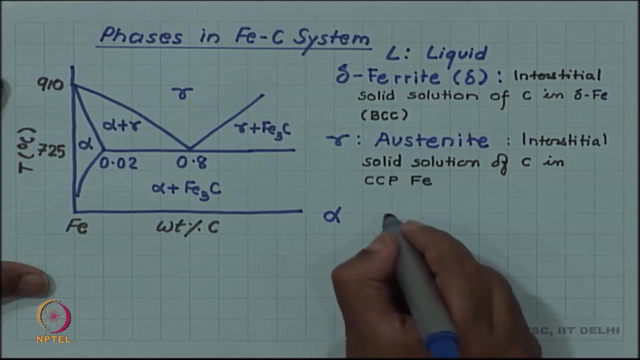 solution: Carbon in CCP, iron, cubic close packed iron, So the structure will be CCP. So this is called austenite, which you see in this part of the diagram. Then you have alpha, which is simply known as ferrite. This is in the lower part of the. 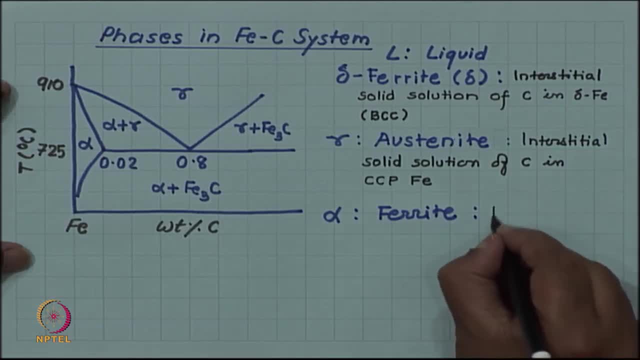 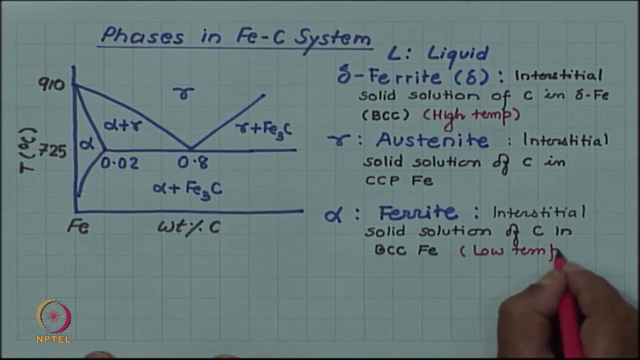 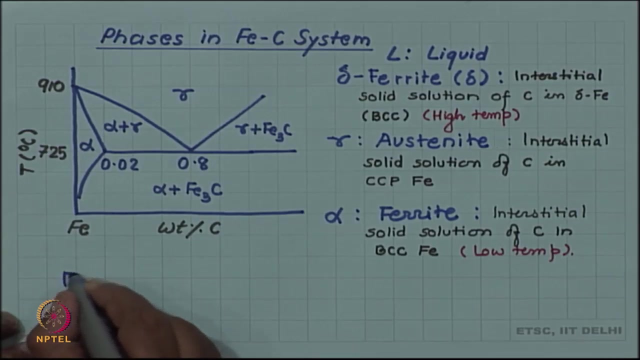 diagram here that is the region of alpha. This is again interstitial. . . . . . �� This is a high temperature version of ferrite. This is a low temperature version of ferrite. And then of course, you have Fe3C which we call cementite. You have to be familiar with 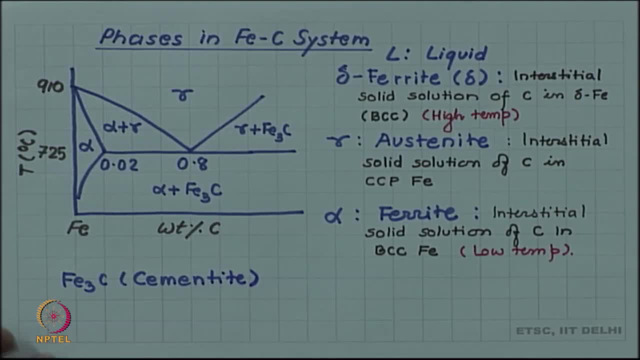 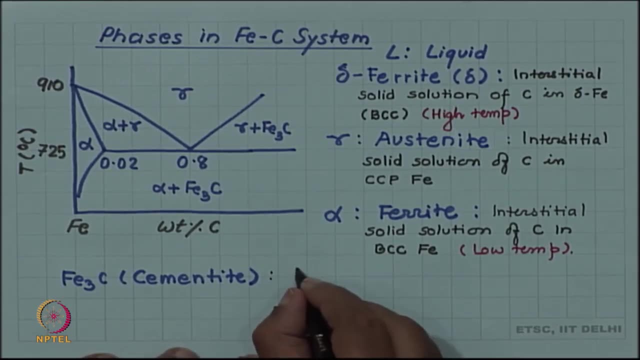 all these for the symbols and the name. these both the symbols and the name, So Fe 3 C, called cementite. this is an intermetallic compound. this is not a solid solution because it have occurs at fixed composition. Fe 3 C. 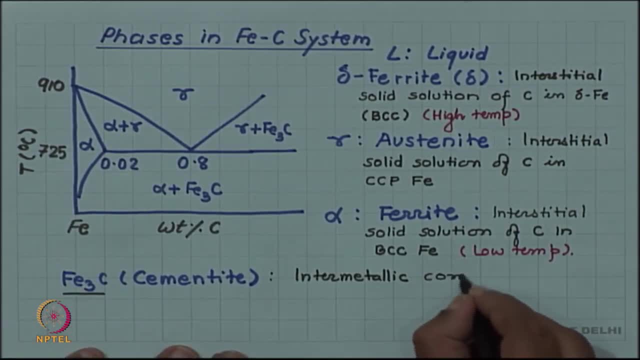 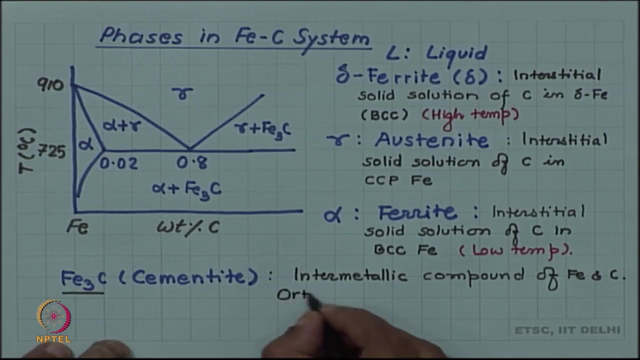 So this is intermetallic compound of iron and carbon. it has an orthorhombic crystal. the crystal structure is complicated. the crystal system is orthorhombic. So we have looked at the phases, the invariant reactions and the various phase boundaries. 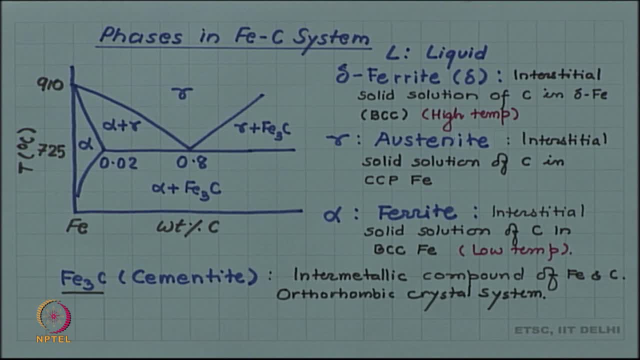 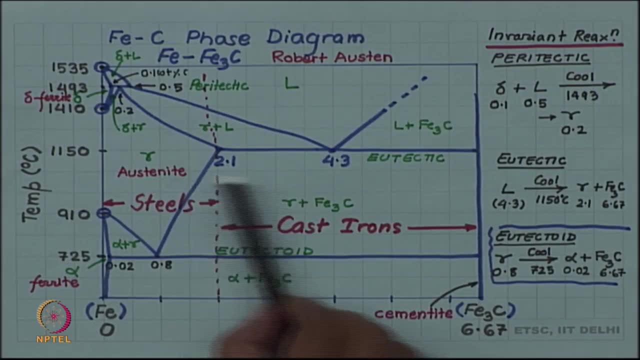 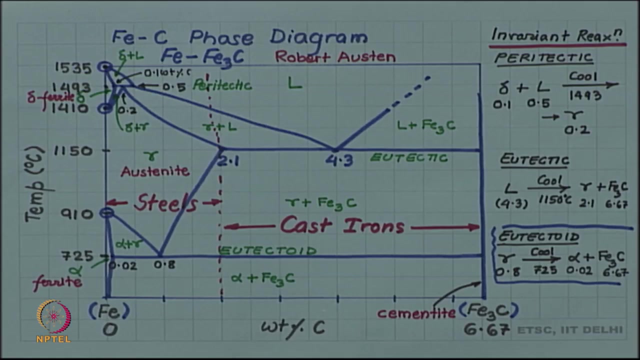 and phase regions in the iron carbon phase diagram. So looked at as a whole, the diagram may look complicated, but just remember that there are three invariant reactions- the peritectic reaction, the eutectic reaction And the eutectoid reaction, and the names of different phases. of course you have to. 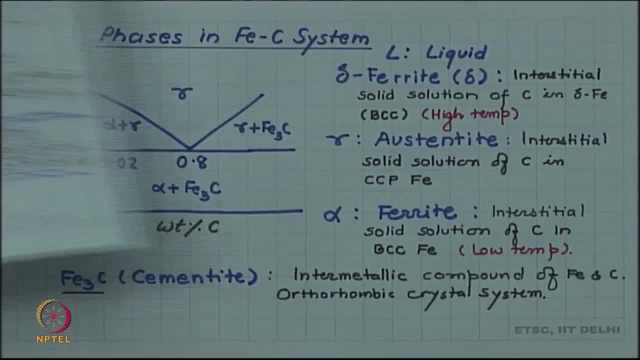 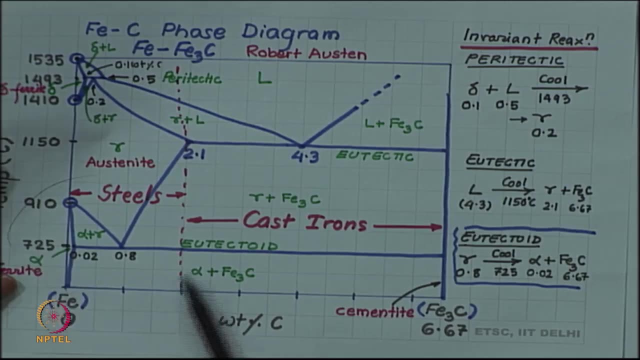 gradually commit them to memory. And then this region of the phase diagram, the low temperature eutectoid region of the phase diagram, is what is important and what we will focus in the forthcoming videos.